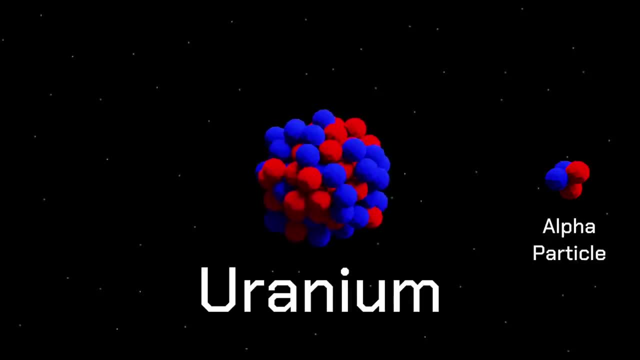 In this process, it gives off heat. This is because we have to respect Einstein's law: E equals MC squared. Energy equals mass times the speed of light squared. This plutonium atom weighs more than the uranium and this alpha particle that was spat out. 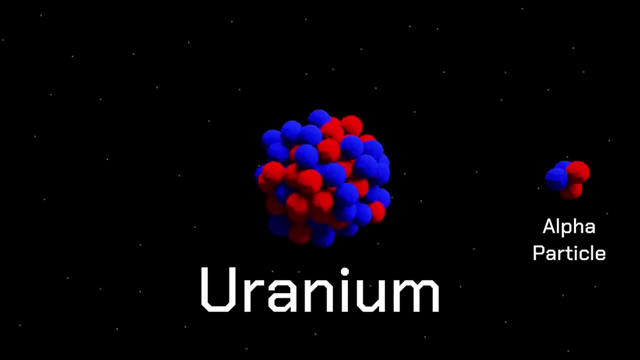 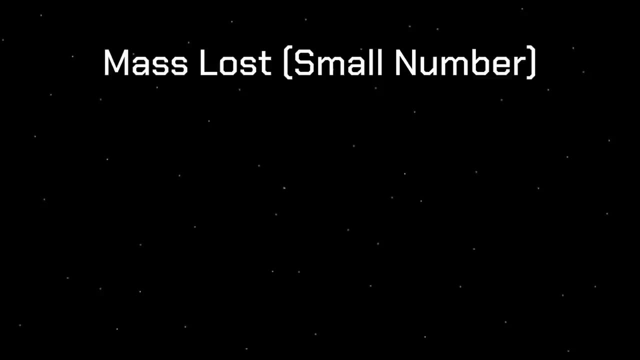 That's because mass was lost when this decay happened. That mass was lost because that mass turned into energy And we take the mass that was lost, multiply it by the speed of light squared, so we get a small amount of mass lost and a huge amount of energy released. 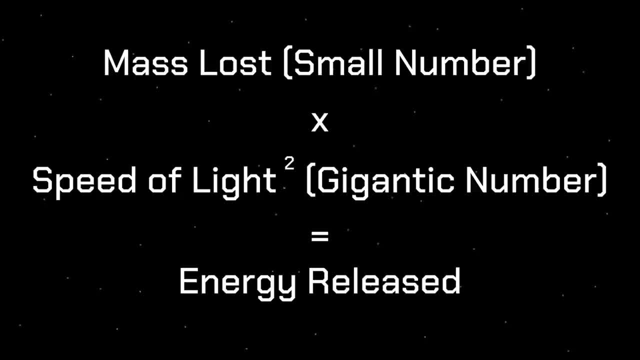 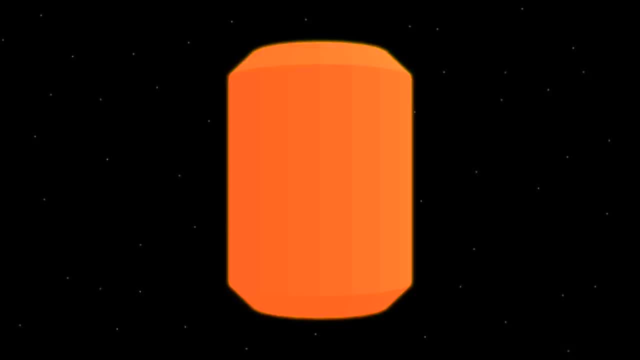 That energy is heat With an absolutely insane weight, With an absolutely insane number of atoms And a chunk of plutonium undergoing this decay. You can quite easily imagine that that chunk of plutonium is going to be quite warm. Now the challenge is converting that heat into electricity that we can use to power our spacecraft. 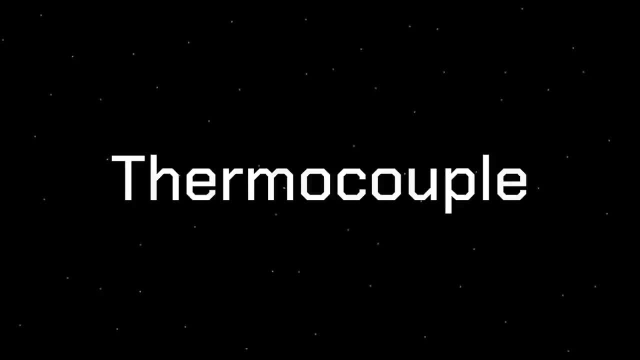 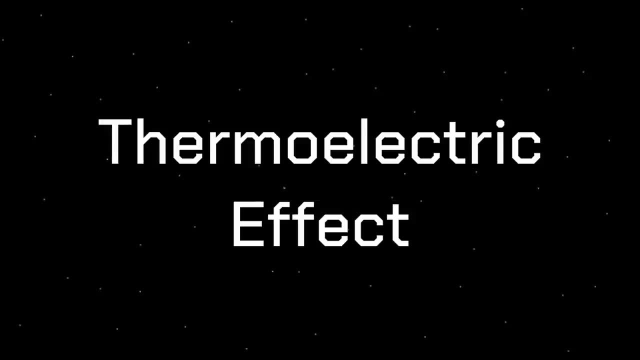 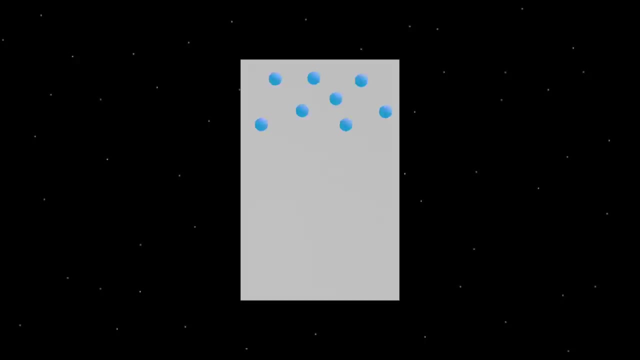 To do that, we are going to be using a thermocouple. Thermocouples utilize the thermoelectric effect, And that means essentially just directly transferring heat energy into electrical energy. We do this by getting a chunk of material called a semiconductor. 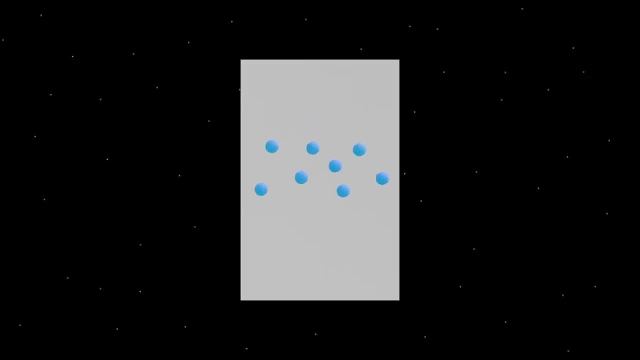 This semiconductor will only allow electrons to flow in this direction. How do we get the electrons to flow? Well, we have to think of what happens to a material when it's warm. Particles in any material, when they're warm, will vibrate. 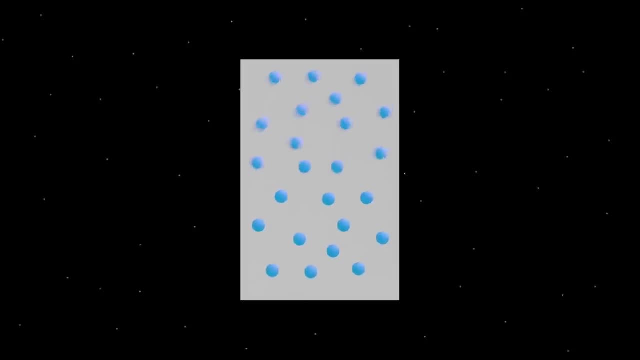 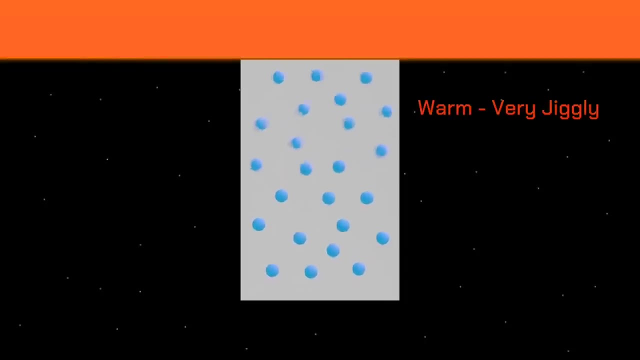 depending on how warm it is. If you warm it up, those particles will jiggle around more. So we see, when we put our semiconductor up to our block of plutonium, we're going to have a warm end and we'll have a cooler end. 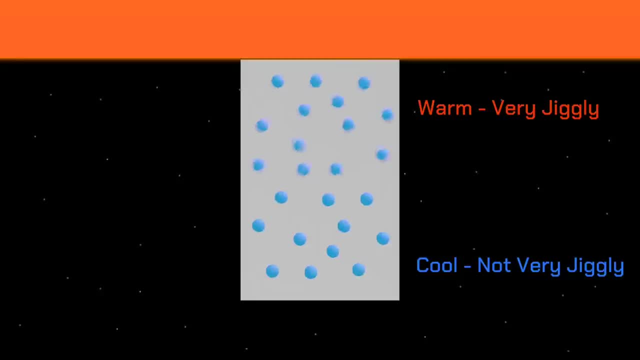 At the warm end, these negatively charged electrons are going to be jiggling about a lot, But at the cold end, not so much. Because of this, these electrons will push their way down to this end of the block of semiconductor. As a result, this end will become negatively charged. 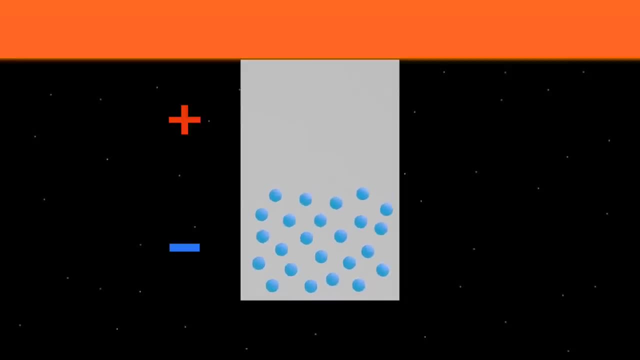 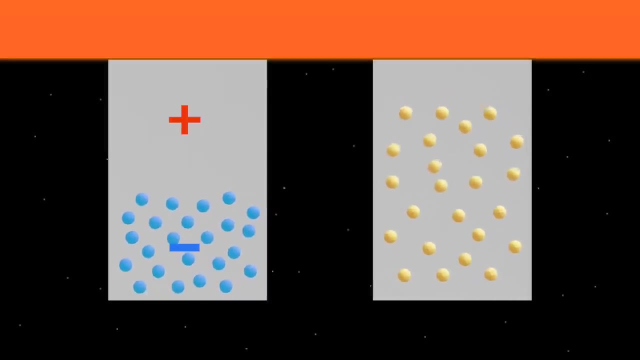 And so kind of like a battery, we'll have a positive end and a negative end. One more along we'll have another semiconductor which will only allow positive charges to move, And so the positive charges will move down in the same way the electron did in the previous one.